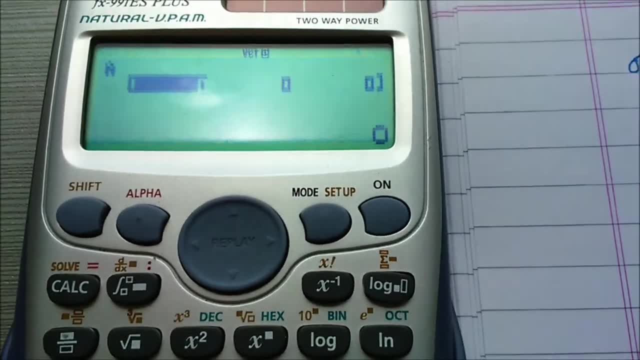 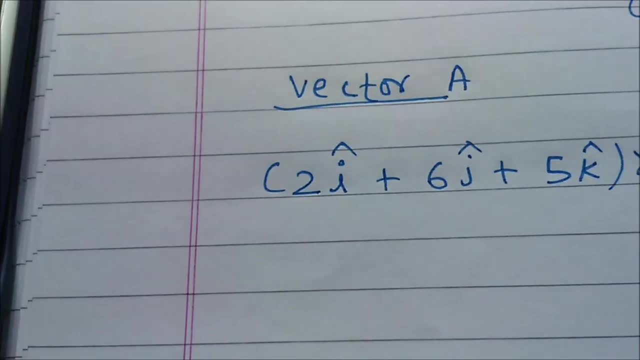 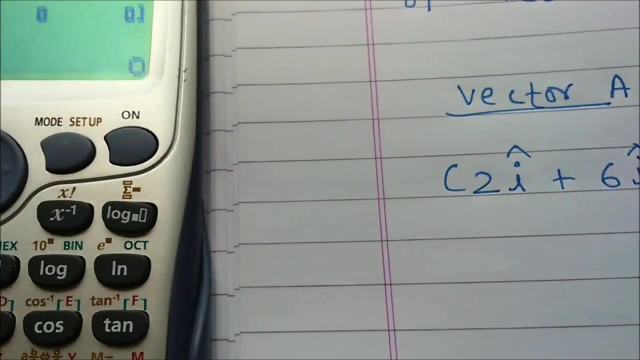 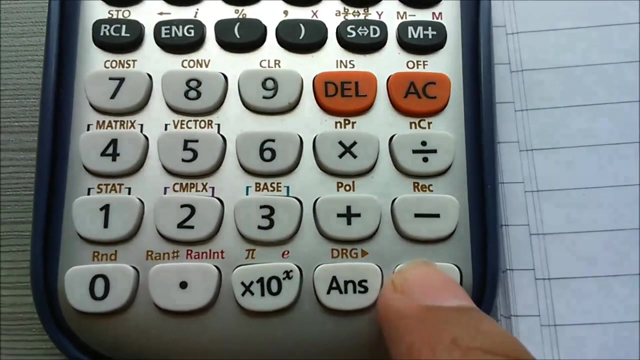 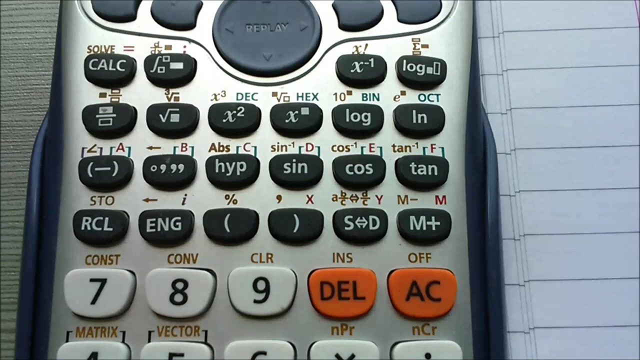 when we pressed one. then we have to give the dimension of the vector a the value of coefficient of i cap, j cap and k. cap is 2, 6 and 5. so fill 2, 6 and 5 here. 2 is equal to 6, is equal to 5, is equal to see. value is loaded: 2, 6 and 5. 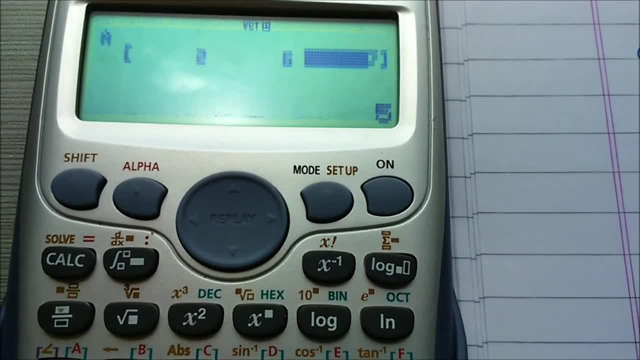 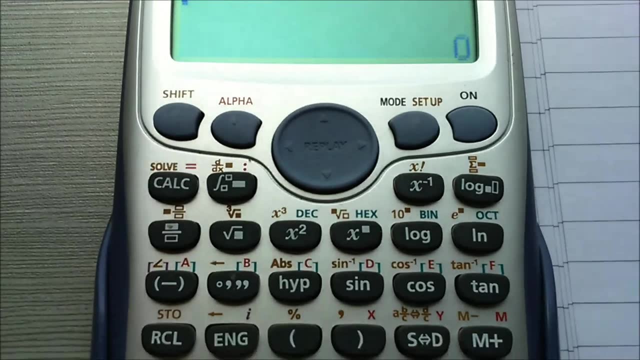 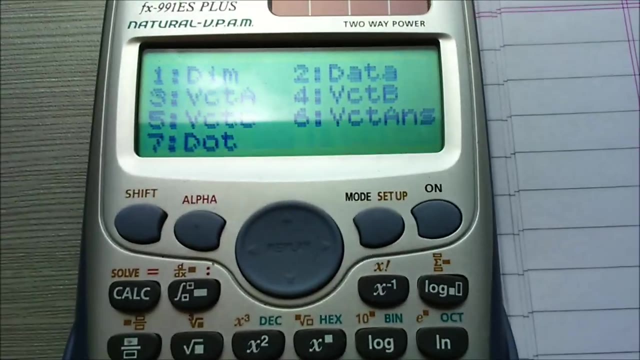 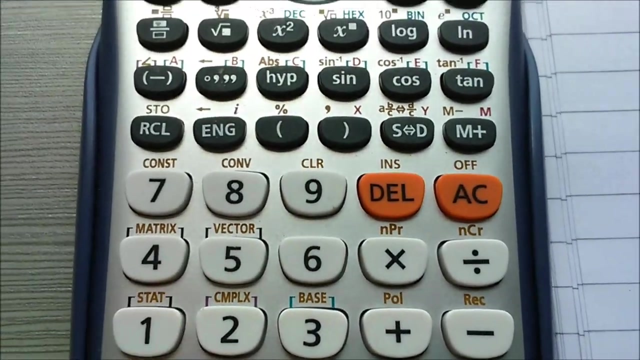 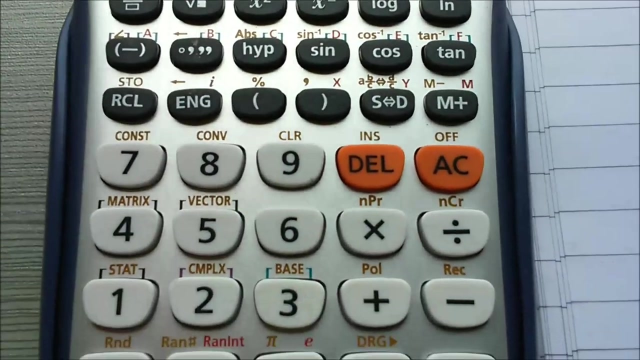 now for loading the value of vector b. vector b: press on button. now press shift and vector is on on number 5. press 5. now give the dimension of vector B. so dimension is on number 1. press 1. vector B is on 2, so press 2. 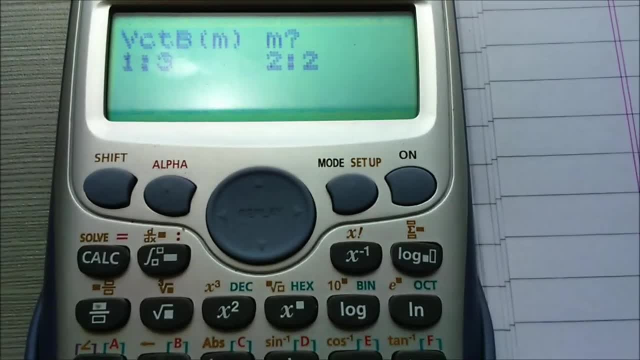 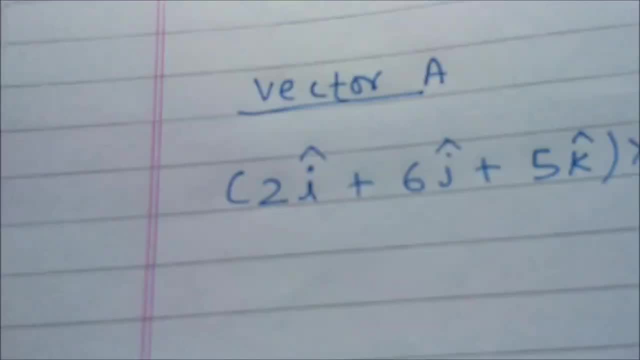 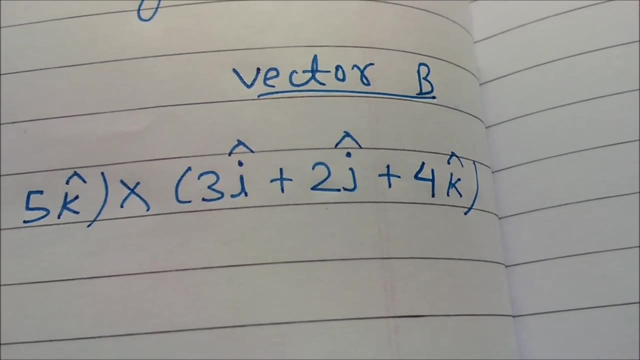 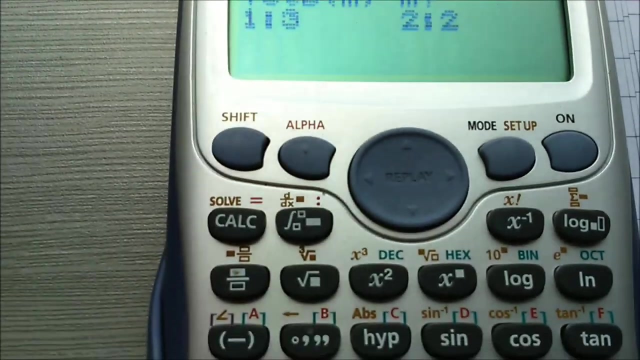 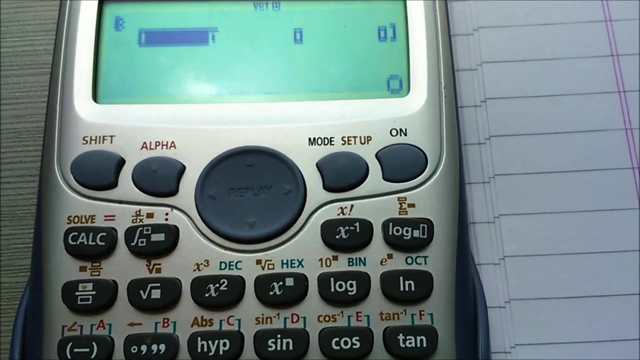 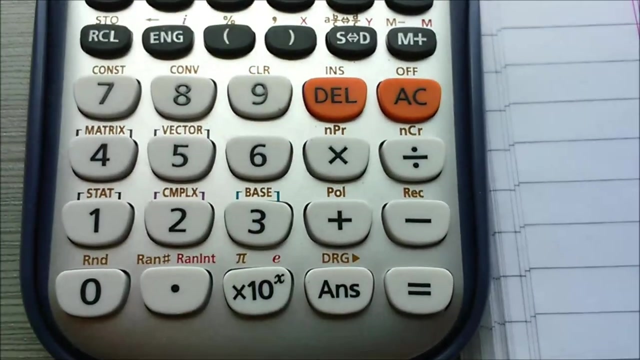 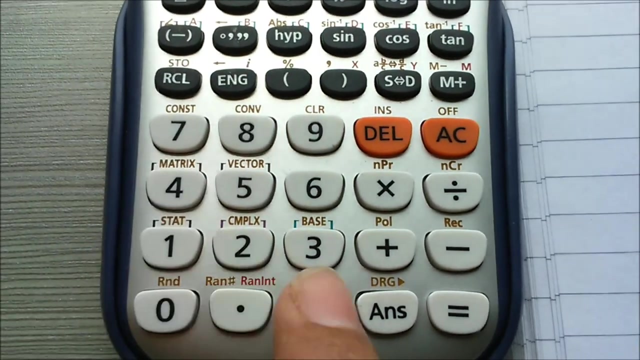 it is a vector B is also of in the three dimension i cap, j cap and k cap. see vector B. also 3 i cap, 2 j cap plus 4 k cap. so values 3 to 4. press 1. now give the. give the values 3, 2 & 4. 3 is equal to, 2 is equal to, 4 is equal to. 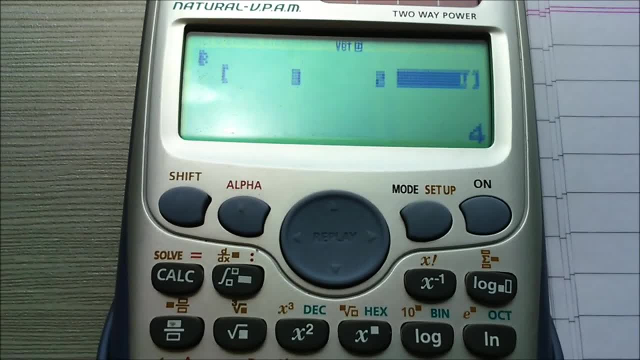 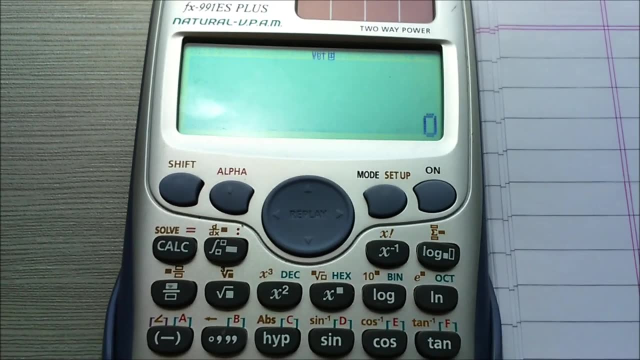 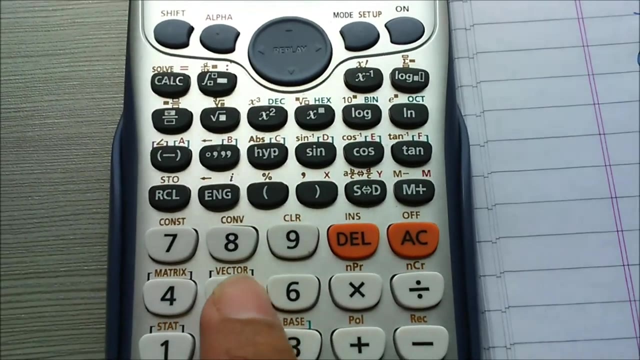 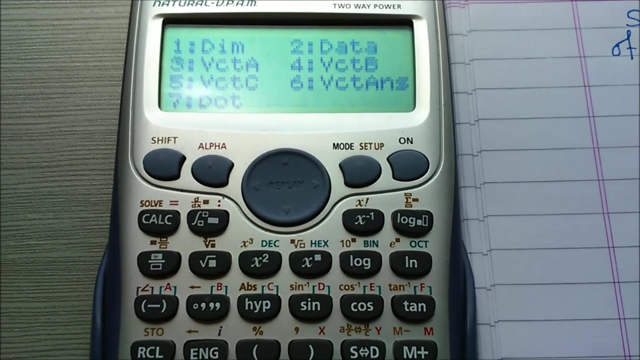 3 to 4 is loaded in the calculator of the vector B dimension now. press on button now. press on button. now for cross product of vector: press shift button and press 5 button. vector A is on 3 and vector B is on 4, so press 3.